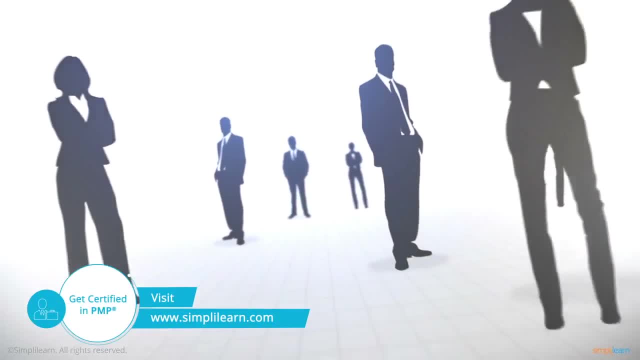 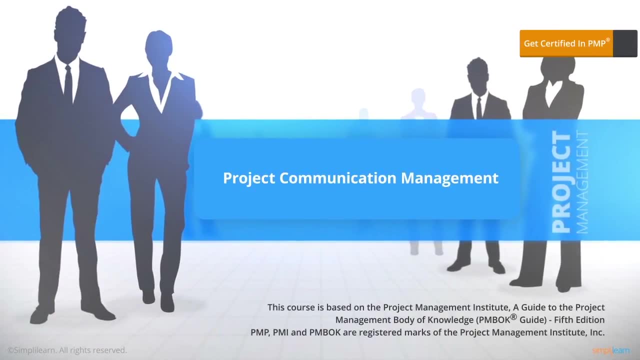 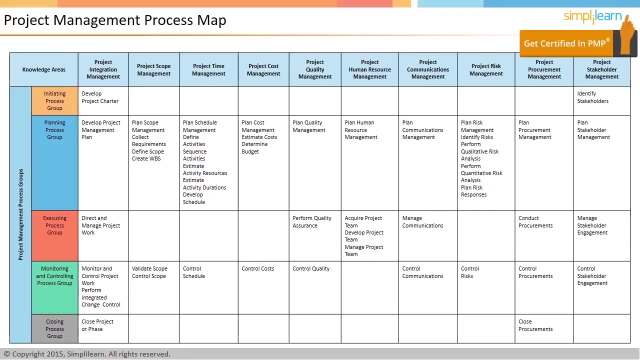 Hello and welcome to PMP certification course offered by SimplyLearn. In this lesson we will focus on project communications management. There are 47 processes in project management, grouped into 10 knowledge areas and mapped into 5 process groups. In this lesson we will look at the seventh knowledge area, that is, project communications management and its processes. 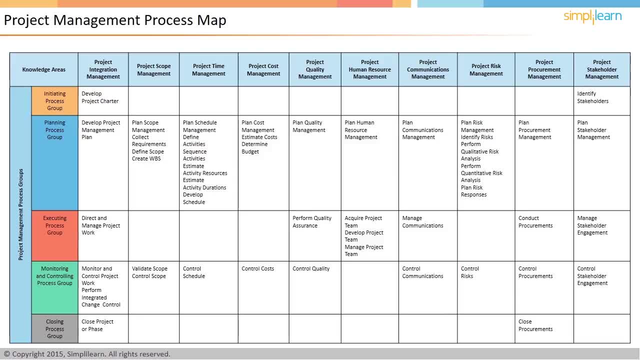 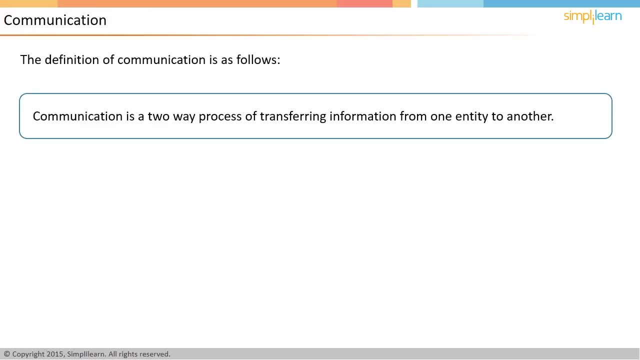 In the next screen. let us understand communication. Communication can be best defined as a two-way process of exchanging information between two entities. As you can see on the screen, if project is an entity, the project needs to communicate with other entities in the organization, like project managers. 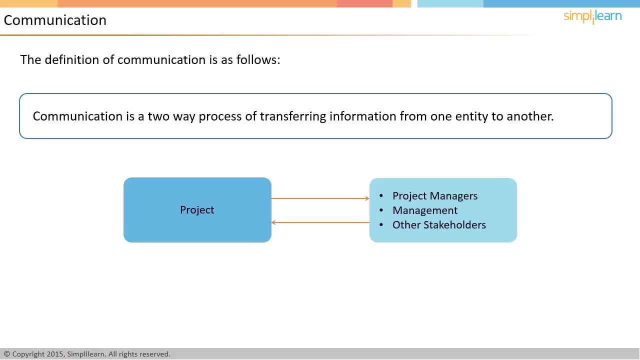 Senior management of the organization and any other stakeholder of the project. Similarly, these entities may also have to communicate with the projects. The communication between project and the stakeholders is always two-sided. Project manager is responsible for ensuring proper communication to and from the project. 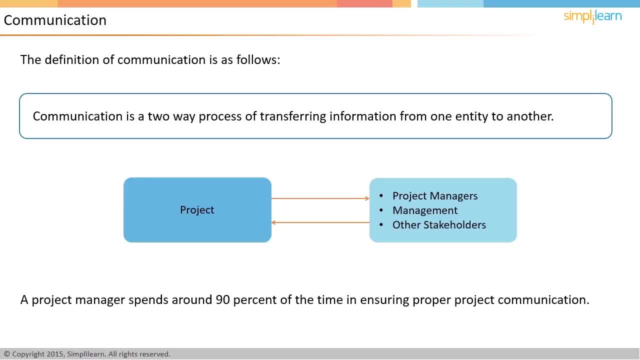 In fact, a project manager spends almost 90% of his or her time on communication. You can now understand how important it is for a project manager to plan this activity well. In the next screen, let us discuss communication methods. Communication can be done in two ways. 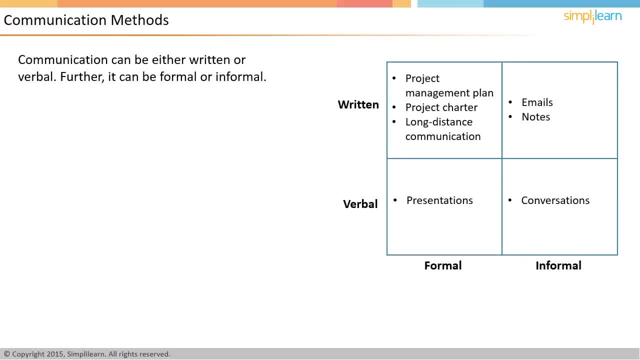 It can be done written or verbal, Both written as well as verbal. communication can either be formal or informal. Formal means communicating by following some basic rules, Whereas informal means taking a course. These two combinations result in four different communication methods. They are formal, written, formal, verbal. informal written and informal verbal. 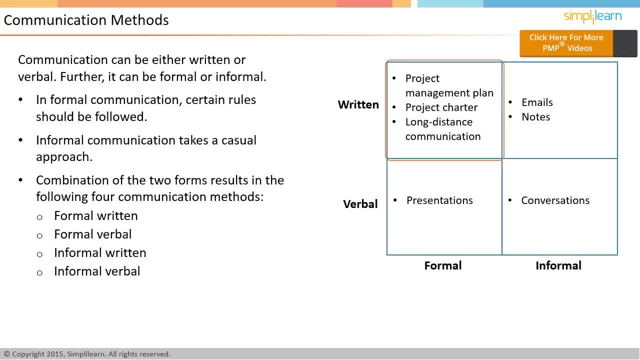 Formal written method is used for project management plans, project charter and over long-distance communication. Formal verbal method is used during presentations, Whereas informal written method is applicable while writing notes or emails. Informal verbal, on the other hand, is applied during conversations. 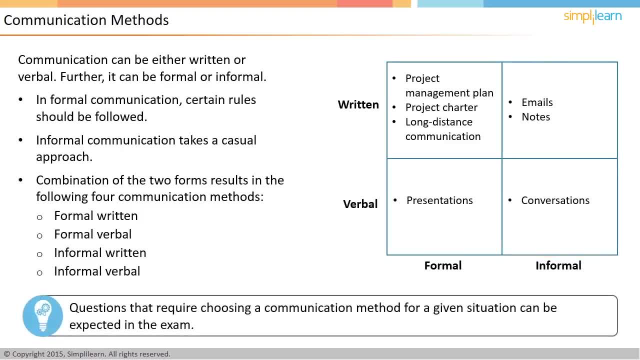 You can expect questions in the PMP exam which require choosing a communication method for a given situation. So a fair understanding of the communication methods can help you score higher. In the next screen, let us look at the various communication technologies. Communication technology refers to the different media used for communicating. 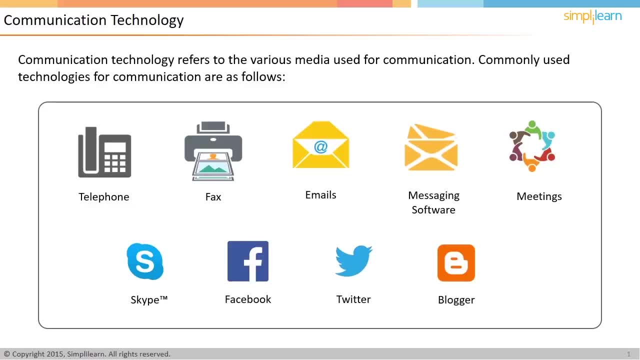 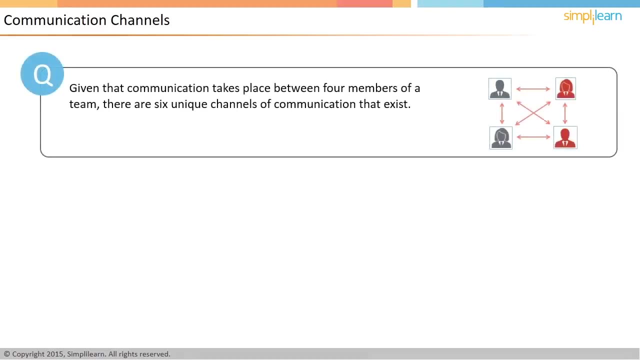 A few such technologies are listed on screen, Among which email, fax and telephone are a few popular communication technologies. In the next screen, let us understand the communication channel with the help of an example. Communication takes place between four people in a team. 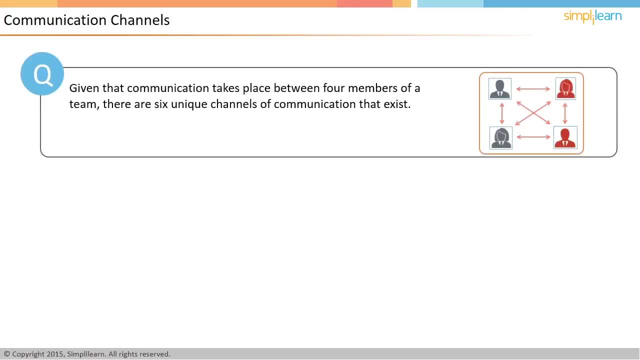 The lines across the members represent there can be six unique channels of communication existing within the team. Now, if the team comprises ten members, how many unique channels of communication will be calculated? You can use the formula n multiplied with n minus one and the resulting sum divided by two. 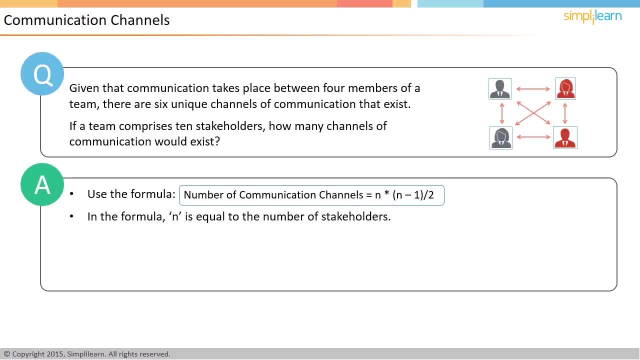 n is the total number of people involved in communication. In this case, n equals to ten. If this is put into the formula, you will get forty-five as the result. Therefore, forty-five unique communication channels exist. It is difficult to manage such a large number of communication channels. 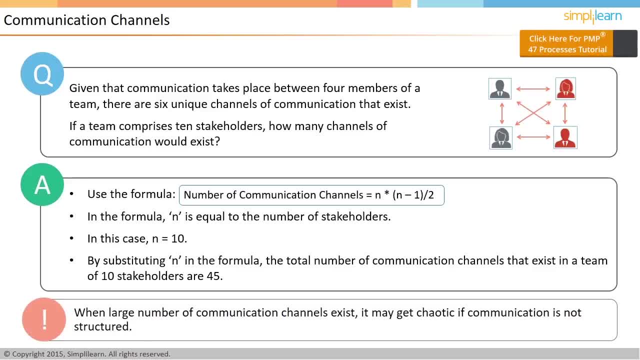 Therefore it is important to structure communication. Otherwise everyone starts communicating everything to everyone and it can become a real chaos in the project. In the PMP exam, you may be asked to calculate the number of communication channels in a scenario-based question.